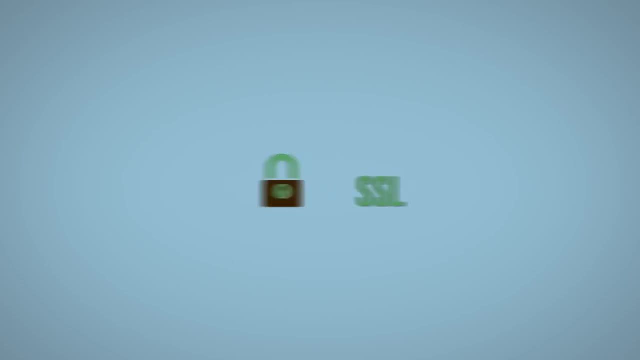 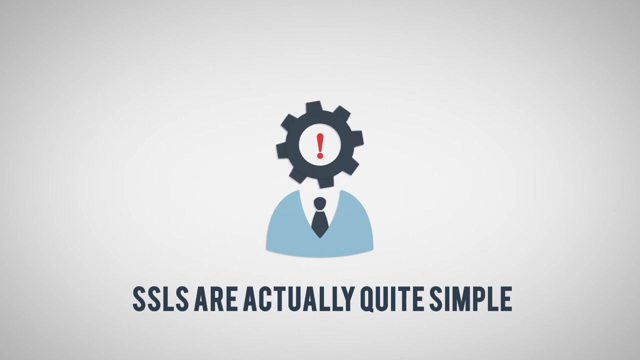 The topic of having an SSL on your website is often raised on business forums and webmaster blogs, Often the subject of much confusion. SSLs are actually quite simple, but yet do have huge potential, good and bad. So what is an SSL and what exactly does it do? 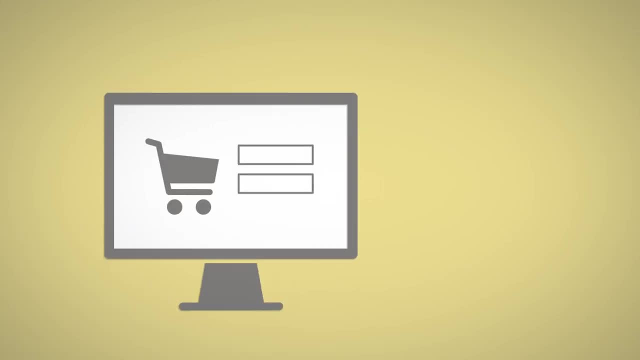 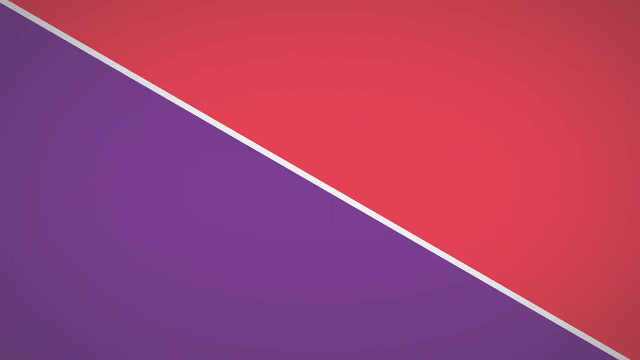 Let's first look at what an SSL does In simple terms. once installed, an SSL encrypts or scrambles information sent to and from your website. The obvious question is: why would you want to do this? The reason, quite simply, is security. 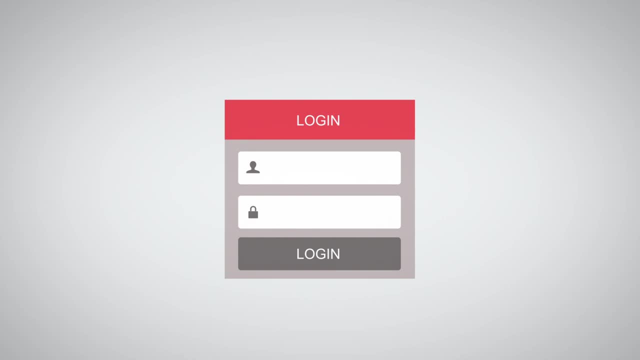 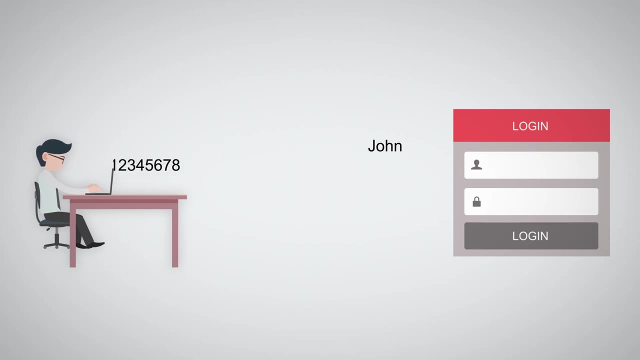 Imagine you have a form on your website. The form may ask personal questions or it might even take credit or debit card details. If someone, for example a customer, completes this form, the data is sent from the user's computer to your website. The data is: 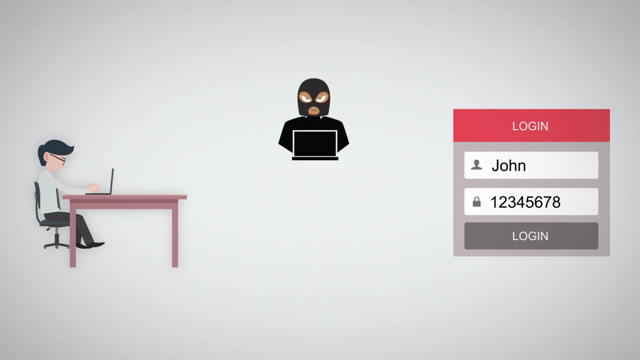 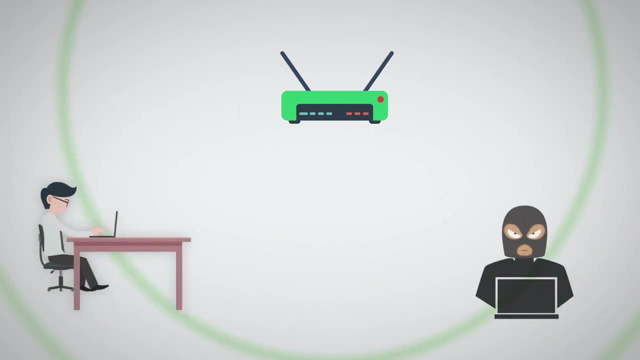 sent pretty much as is. However, if someone- a hacker for example- wished to intercept this data, they potentially could. In fact, this would be as easy as being within range of the user's Wi-Fi router with some free software installed on their laptop. Once they run the software and 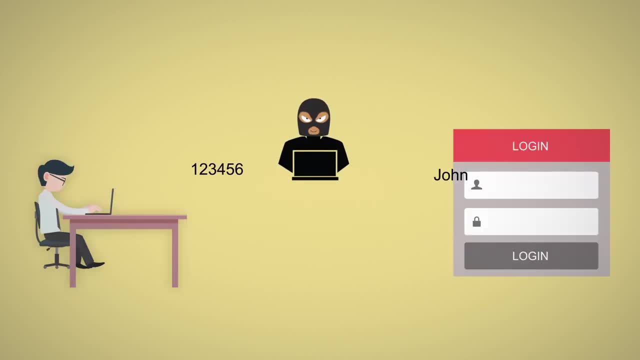 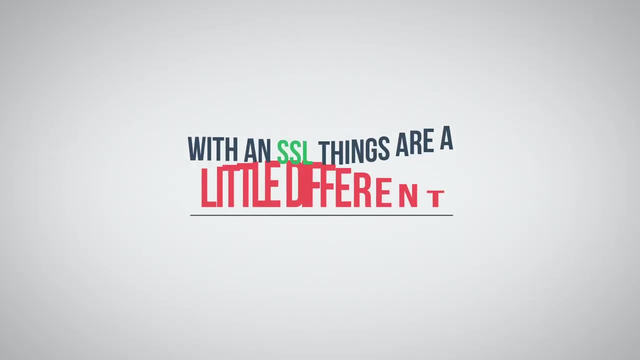 intercept the data, they would very easily be able to read it. Obviously, if this data includes credit or debit card details or passwords, this is a major security concern. However, with an SSL, things are a little different. A hacker could still intercept the data, but it would be completely. 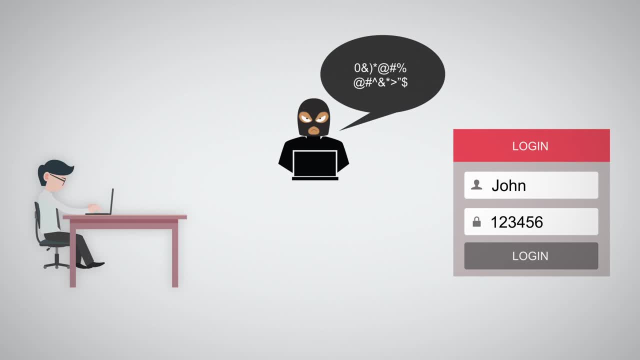 unreadable to them Because of the encryption applied by the SSL. the data is converted into complex code at the user's end and decoded back at the website's server. At the point the hacker could intercept over Wi-Fi, the data would be unreadable. 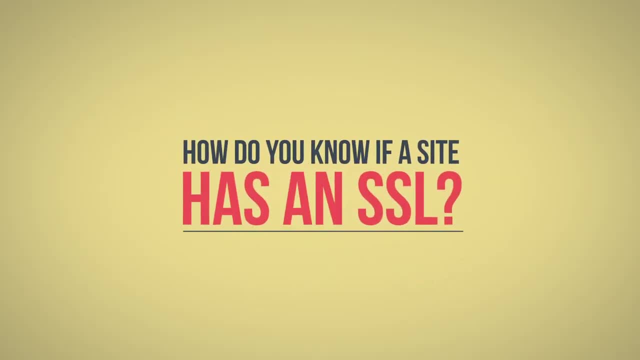 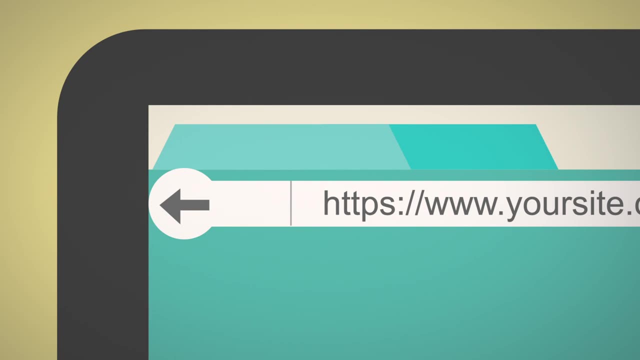 So how do you know if a site has an SSL? There are a couple of ways you will know this. Most web browsers will display a small lock or padlock icon if you're viewing a secure site. This is your web browser's way of letting you know you're viewing a secure site. 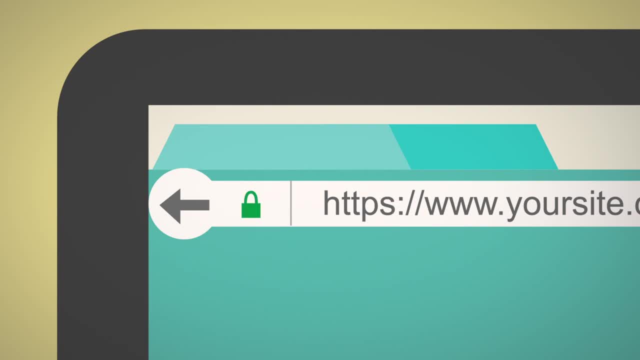 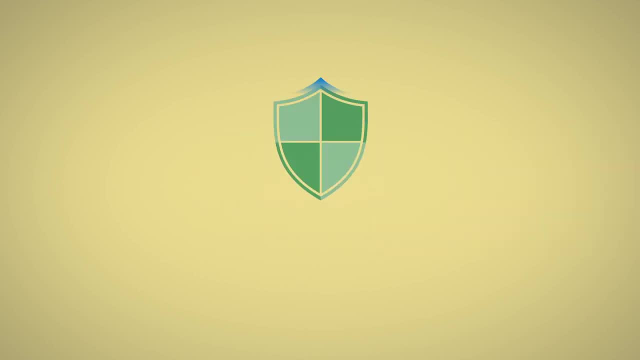 The address of a secure website will start with HTTPS rather than HTTP. Do users care? Overwhelming evidence suggests that they do care. The confidence of knowing a website is protected by an SSL allows users to enter personal information without the worry of that data being insecure. Showing your customers.